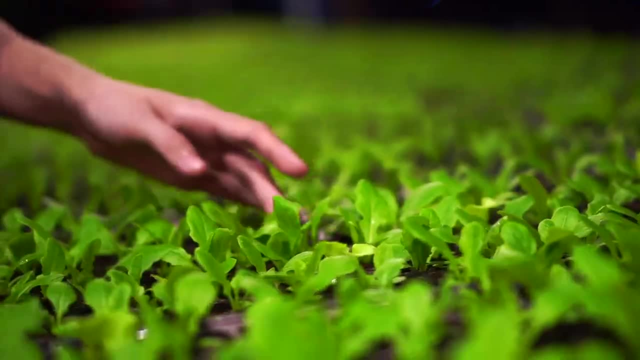 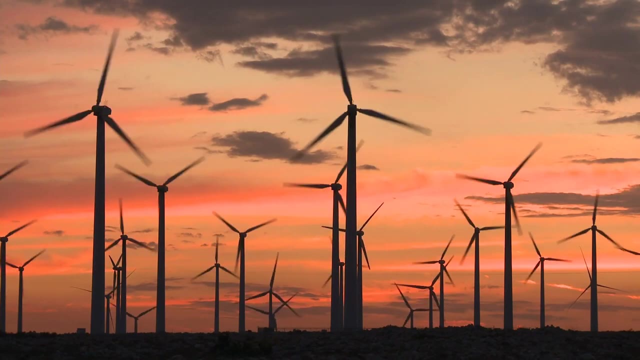 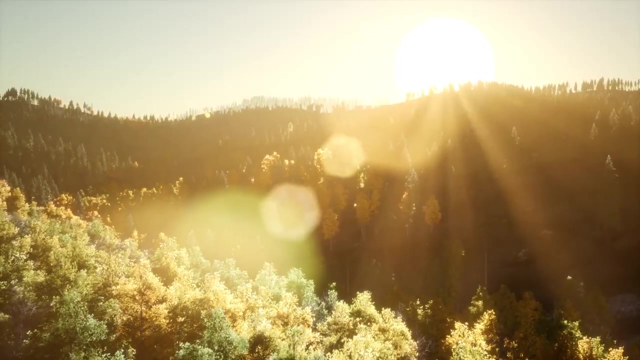 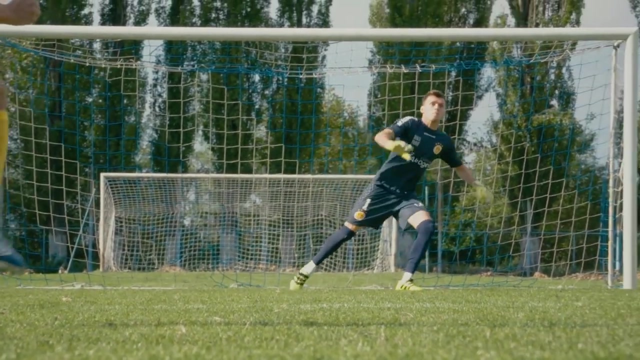 Plants and other organisms need energy to live, grow and carry out life processes. Energy cannot be created, nor can it be destroyed, but it can be changed or transformed from one form to another, And we can observe this happening around us. Let's take a look at some examples. As each video plays, write down the energy transformations. 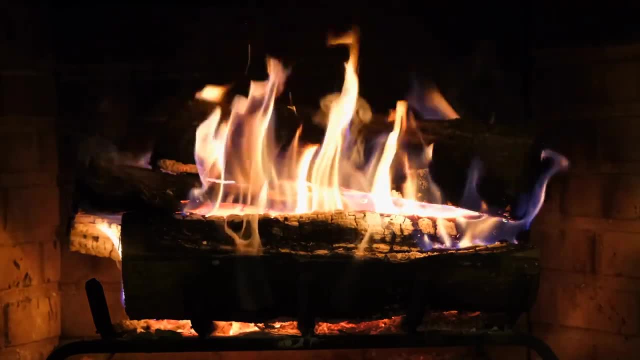 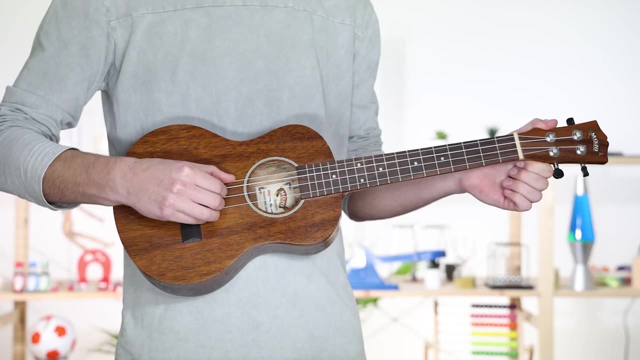 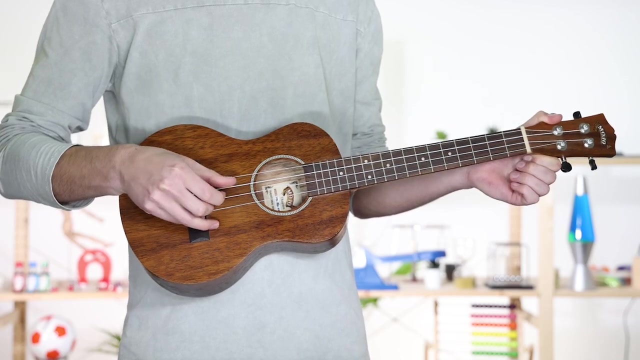 you think are taking place. We'll go through each example at the end so you can check your answers. Let's go. 1. What energy transformation takes place when a ukulele is strummed? 2. What energy transformation takes place when a light bulb is switched on? 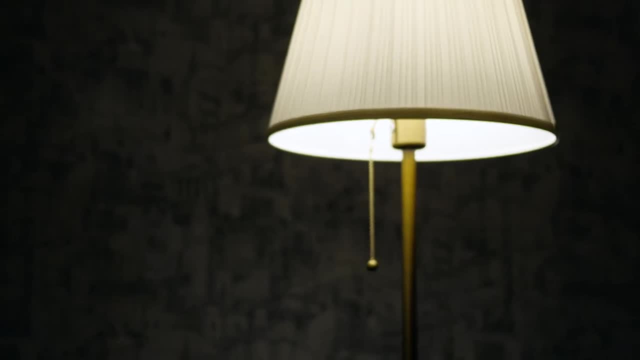 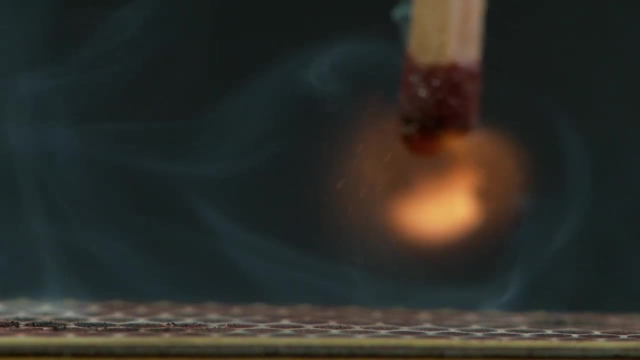 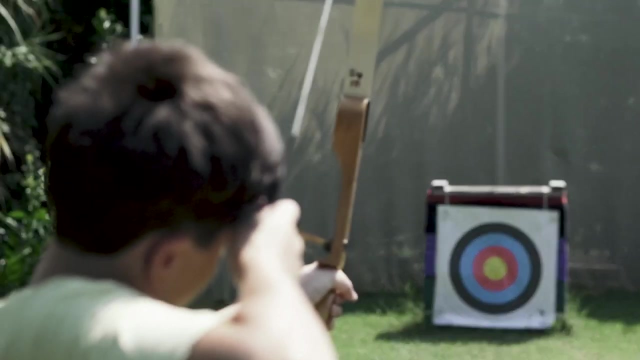 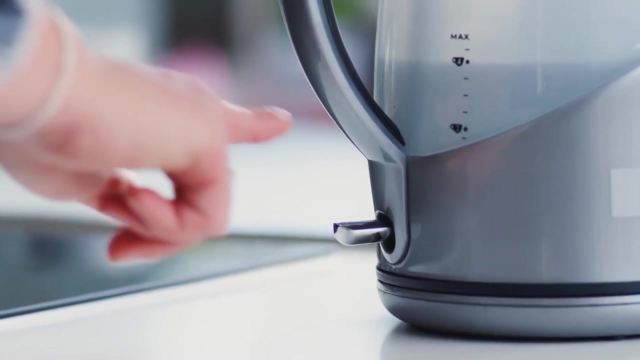 3. What transformation takes place when a match is struck? 4. What transformation takes place when a drawn bow and arrow is released? 5. What energy transformation takes place when a light bulb is switched on? least number five: what transformation takes place when an electric kettle is switched on? 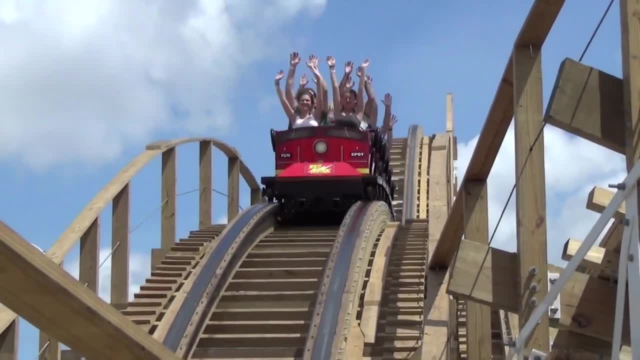 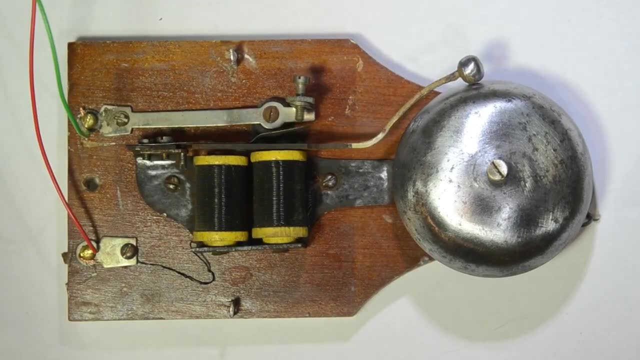 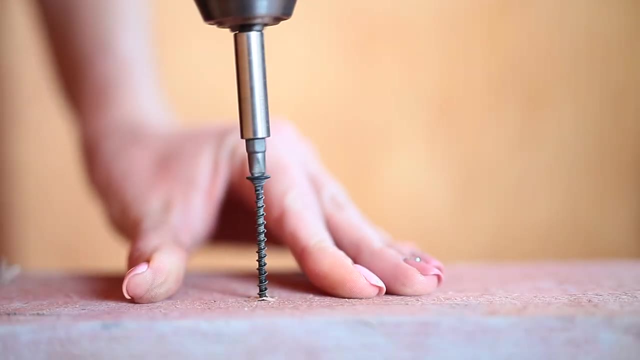 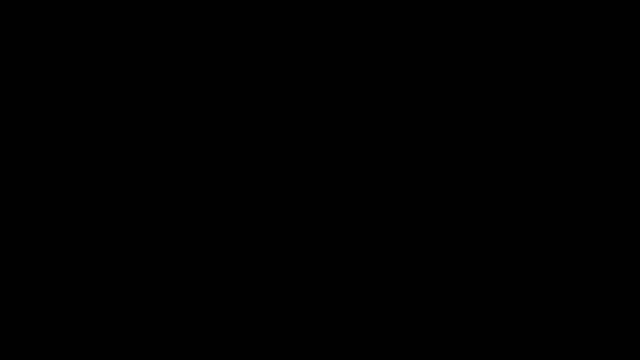 number six: what energy transformation takes place when a roller coaster rolls down the track? number seven: what transformation takes place when an electric doorbell is pressed? number eight: what energy transformation takes place when a drill is used to secure a screw into wood? how'd you go? let's take another look. 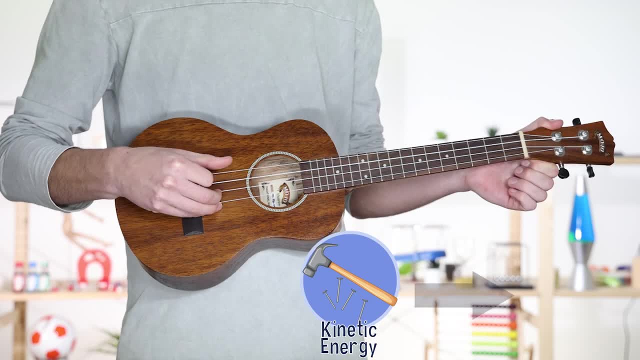 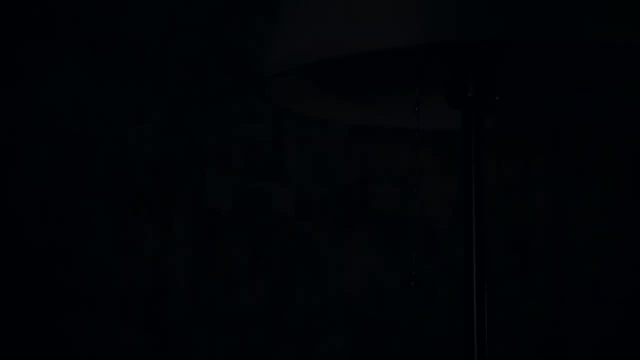 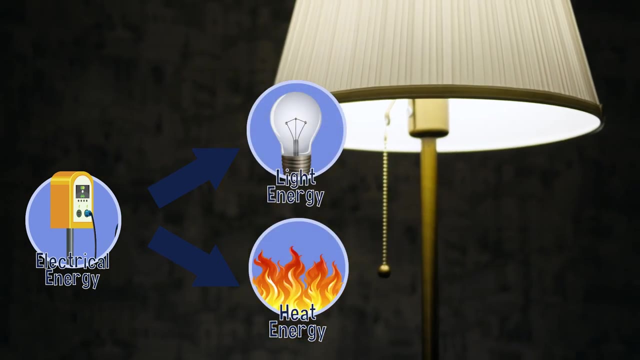 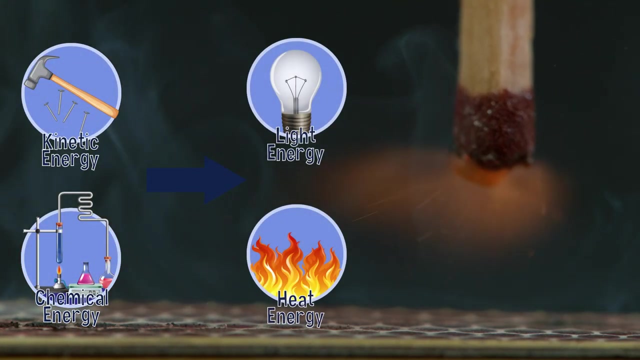 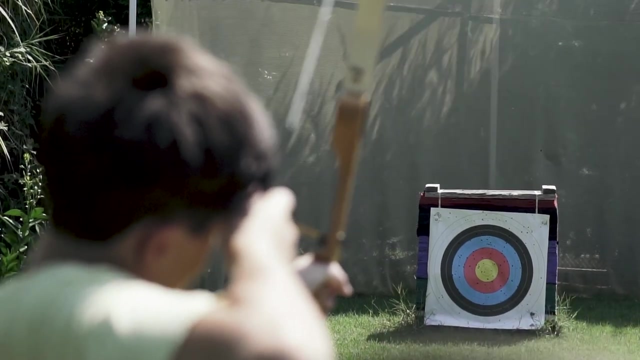 when a ukulele is strummed, kinetic energy is transformed into sound energy. when a light bulb is switched on, electrical energy is transformed into light and heat. when a match is struck, kinetic energy and chemical energy is transformed into light and heat. when a drawn bow and arrow is released, elastic potential energy is converted into kinetic energy.